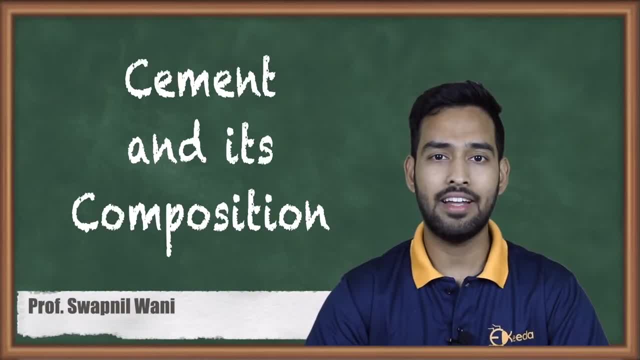 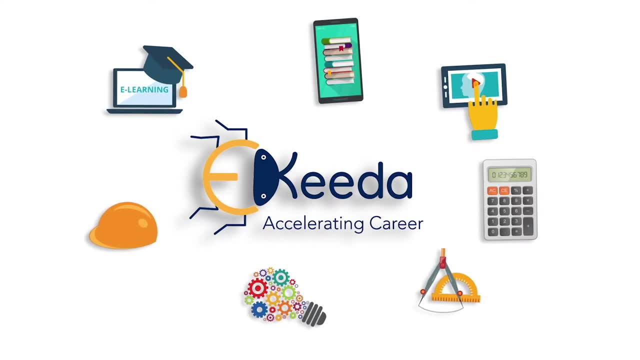 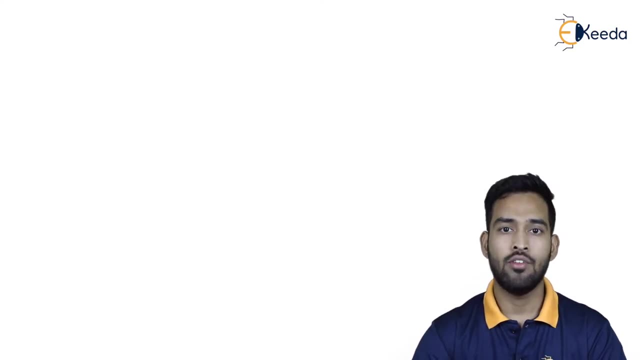 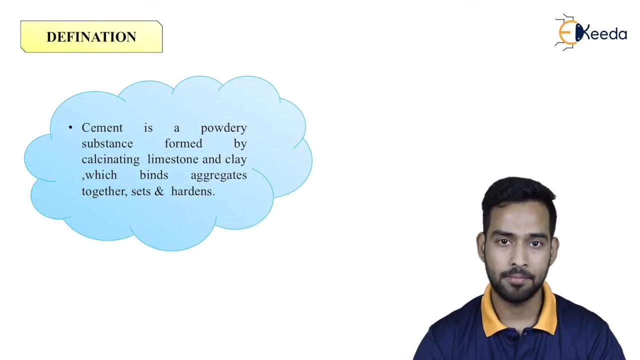 Hello friends, in this video, we will be discussing about cement and its composition. Cement, which is the most important material in the construction industry, which is formed by using different components. Now, what is the definition of cement In exact word? as we discussed, cement is a powdery substance formed by calcinating limestone and clay, which binds. 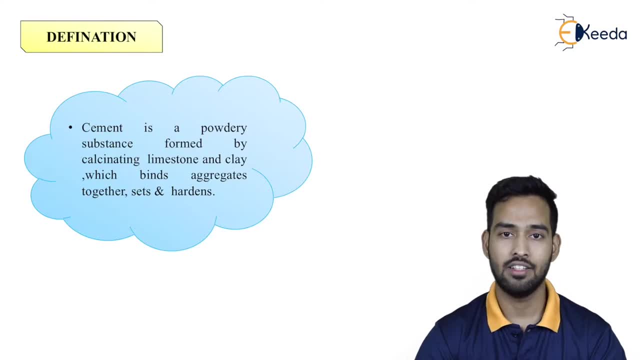 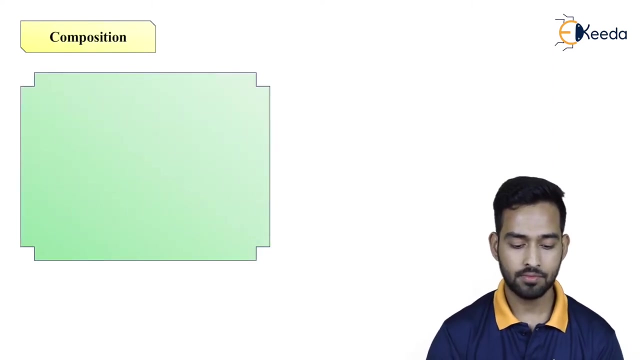 aggregates together, sets and hardens. So cement, as you can say, it, is a binding agent which binds aggregates together and it will set and harden, and it is formed by calcinating limestone and clay. In further slides we will discuss about the combinations of cement. In cement, we require raw material. 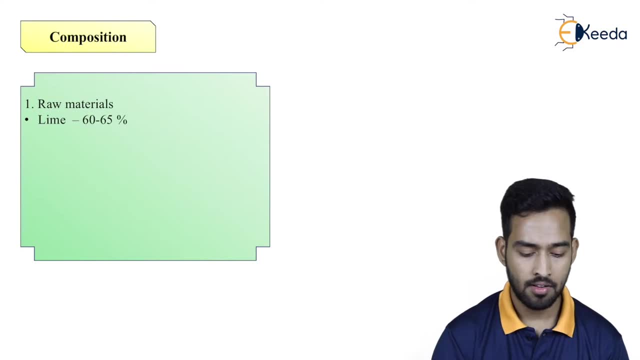 which is lime. Lime is the main raw material in the formation of your cement, which is above 60-65%. Silica is placed between 17-25% and alumina 3.5-9%. Iodine is placed between 17-25% and alumina 3.5-9%. 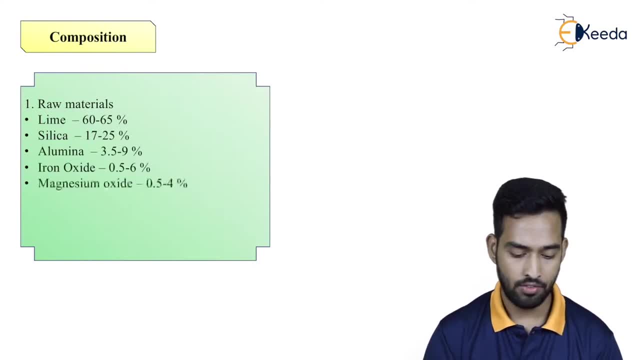 Iodine is placed between 17-25% and alumina 3.5-9% Iodine is placed between 17-25% and alumina 3.5-9% oxide- 0.5 to 5 percent. then we have magnesium oxide, which is about 0.5 to 4 percent, and 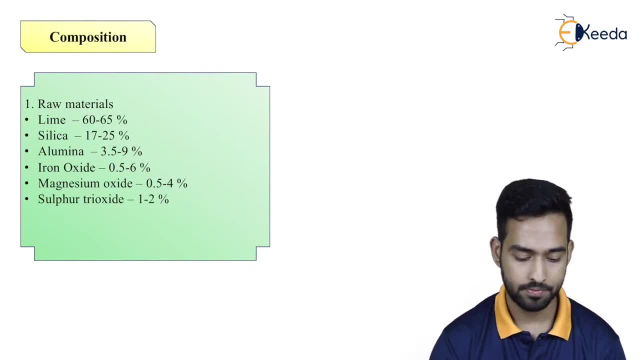 sulfur trioxide, which is 1 to 2 percent. and last is alkalis, generally in the form of 0.5 to 1.3 percent. so from this we can see lime, silica and alumina plays very important role in the manufacturing of cement and these are the main components of your cement. so lime, take already 60. 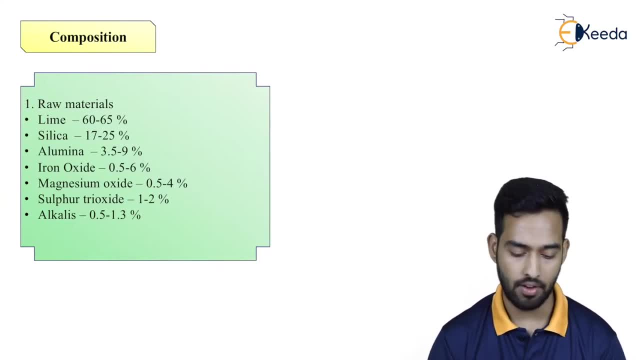 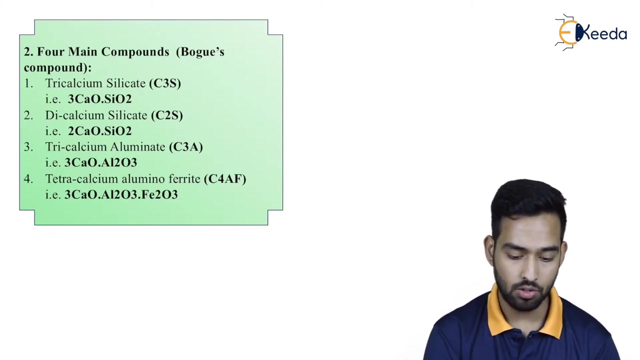 to 65 percent, silica 17 to 25 percent and gypsum might be present in the amount of 0.2 percent only. let us discuss about the four main compounds. that is also known as your bogies compound, and these are very important and their properties we should be understand before using the cement. 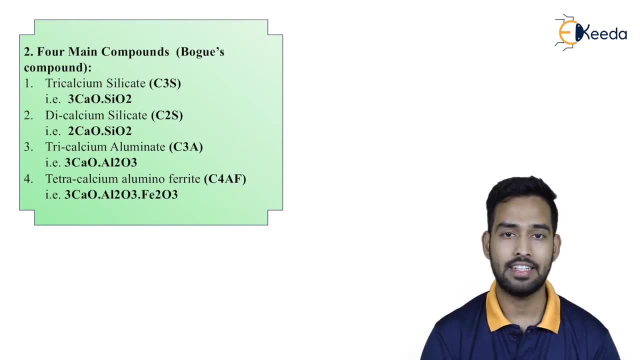 the first compound is tricalcium silicate, which is also known as c3s. that is nothing but 3cao si o2, so remember tricalcium silicate, c3s. next is dicalcium silicate, that is c2s. 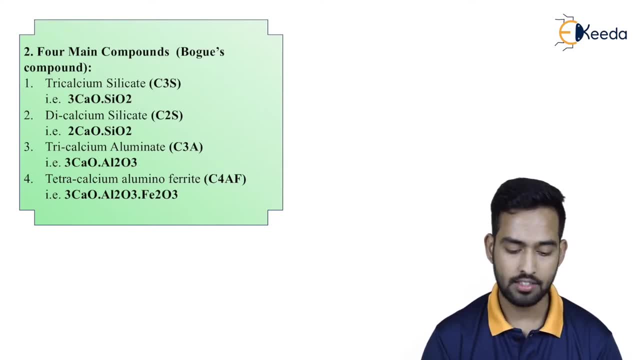 and its chemical formula is 2, 0.6 cao, si, o2. third is tricalcium aluminate, that is c3a, that is c3cao, l2, o3. and last is tetra calcium alumino ferrite, which is c4af. these are the main four components of cement, which is c3s, c2s. 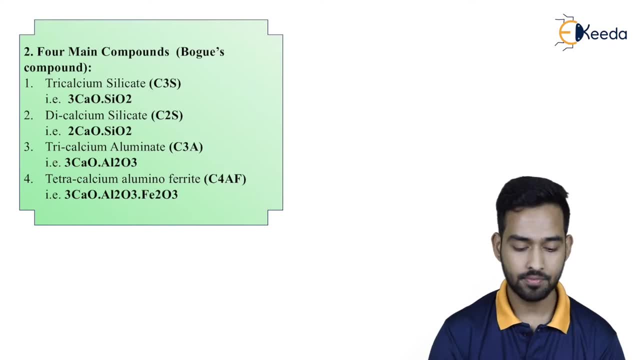 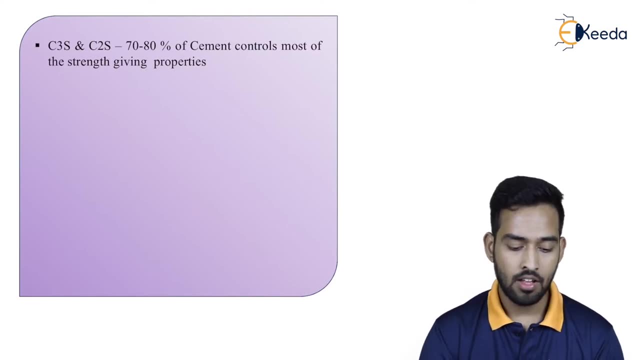 c4a and c4af. i will discuss about effects of these compounds on cement properties. c3s and c2s are generally 70 to 80 percent of cement control. most of the strength giving properties- the most of the strength giving properties- are controlled by c3s and c2s. 26 Ft2rc4 C3Ps also commands a coil structure within the sort H2O'rleth C3 s- often consists of due to similar��s as as 0.6mg in tank or single columnقةic and inil amyloprimate, and also contains a lot of hydrocarbons. 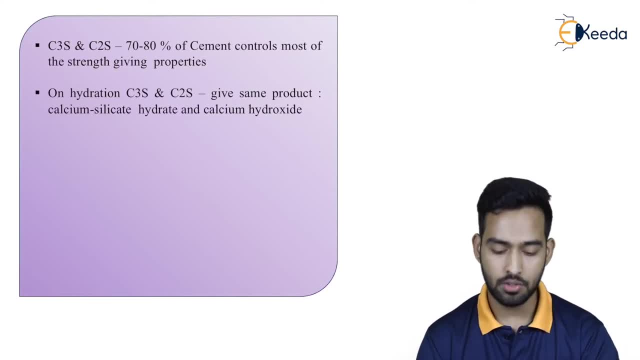 C4a, Ft6s, Ce2s, ACS cumulates jonganolinarly and has لا base sorgen coaching components on the Lynx equation On hydration. C3S and C2S give same product, ie calcium, silicate hydrate and calcium. 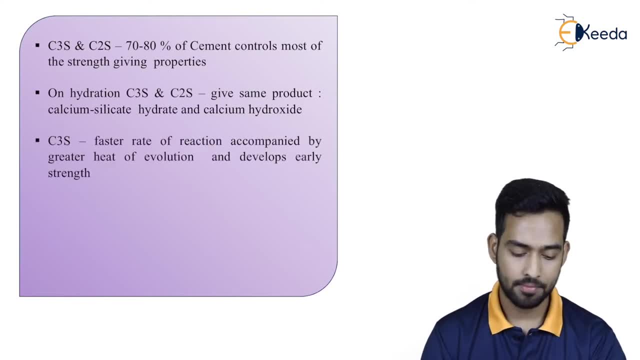 hydroxide. C3S is faster rate of reaction, accompanied by faster or greater heat of evolution, and develops early strength. So C3S is responsible for early strength. So we will keep in mind C3S is important for early strength. It means what? 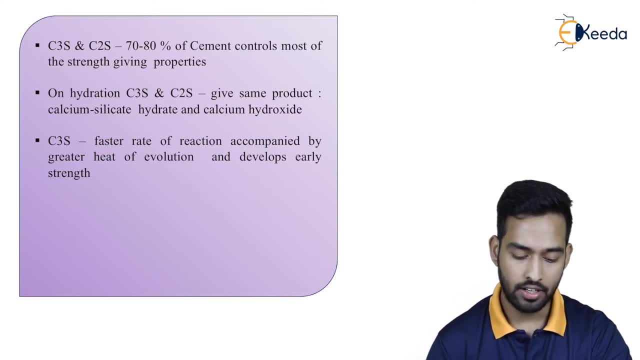 It will give higher rate of heat of hydration. C3S liberates nearly three times as much as calcium hydroxide on hydration as C2S, So C3S will give out three times more carbon dioxide or carbon hydroxide As compared to your C2S, whereas C2S hardens slowly and provide much of the ultimate strength.